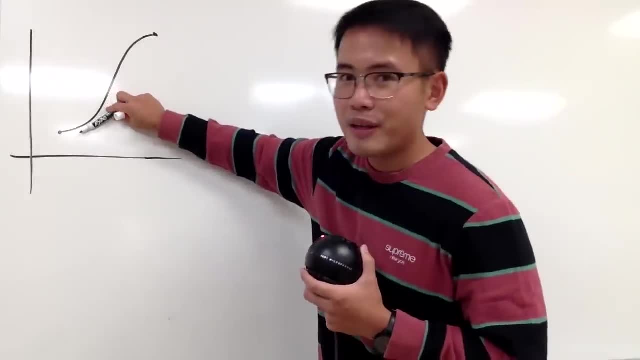 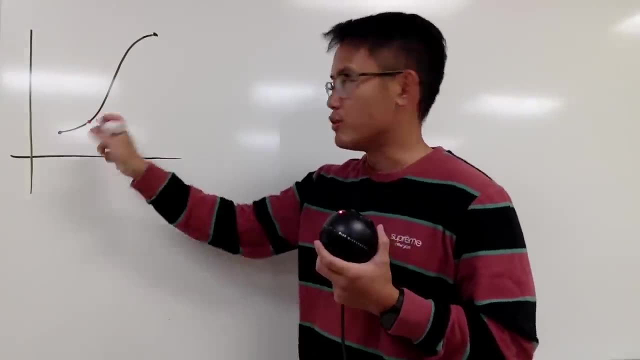 Because, imagine, this is a ruler. you have to just place the ruler right here and what do you get? A tangent line: Excellent, So here's the deal. Maybe I'll just pick a point for demonstration right here and I'm just going to draw a little tangent statement like this: 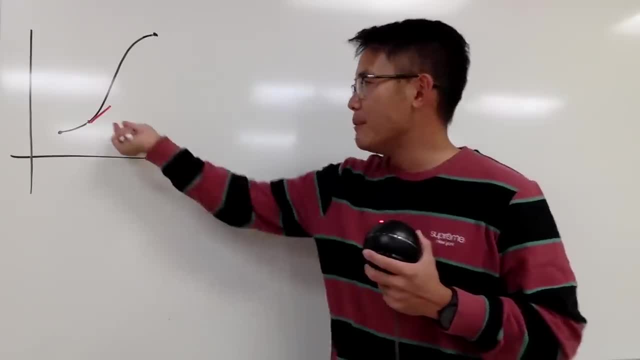 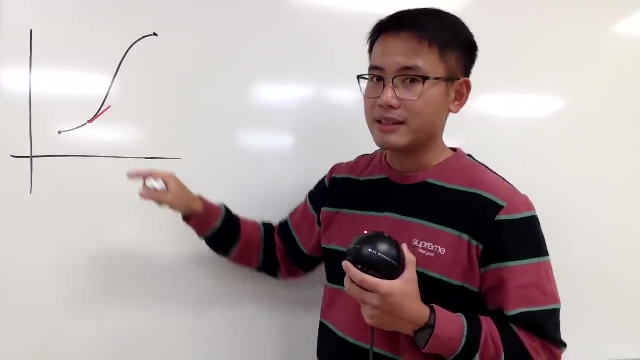 And this right here is supposed to be really, really small, but if I make it so small nobody can see it, so I will just have to make it big. And the idea is that this right here, this length, we can calculate it, and this length is going to be really really close to this. 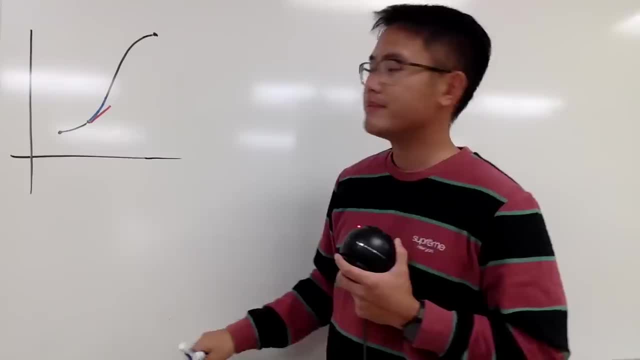 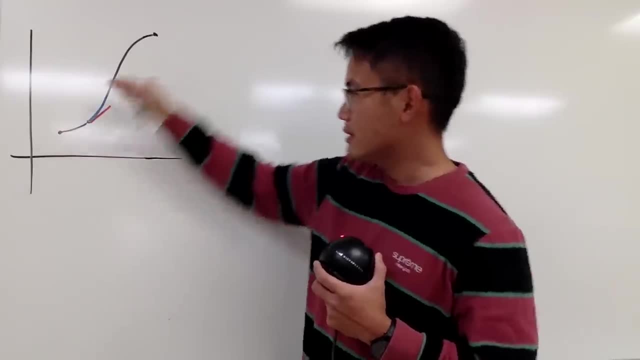 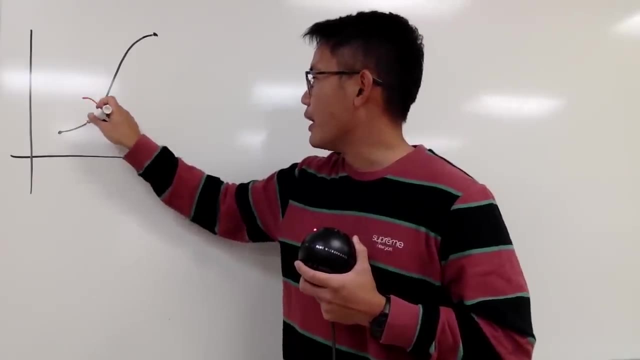 and we'll be using the red part and we'll be using the red part to approximate the blue part and then we'll just add up all the such red part. then we'll get the arc length. That's pretty much the idea. All right For this. right here I will call it to be dl. Some books call it to be d little. 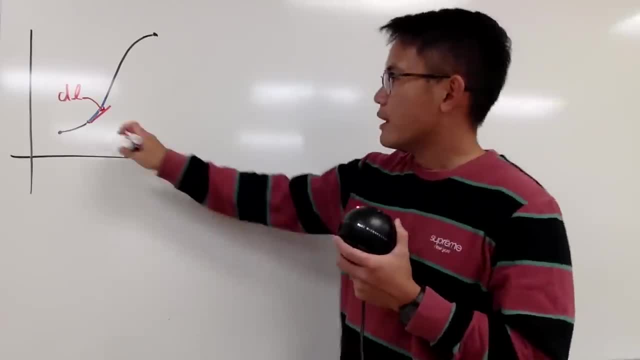 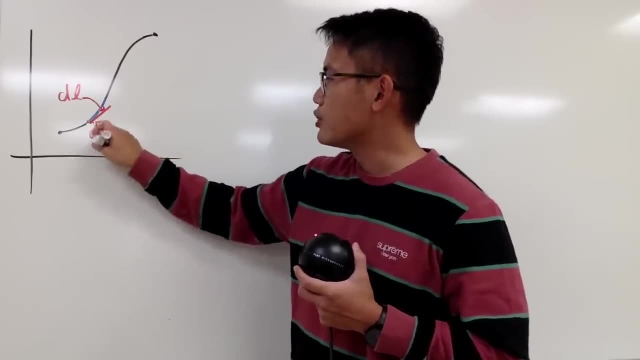 s. Well, it doesn't really matter. Well, here's the deal. I will actually look at this and I'll go horizontally like that, because this right here is the small change amount in the x values, that's dx, And then I will. 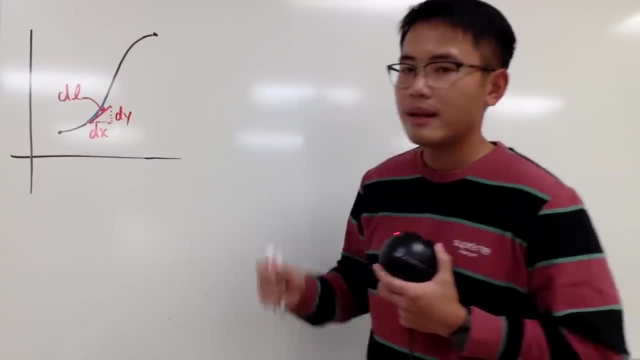 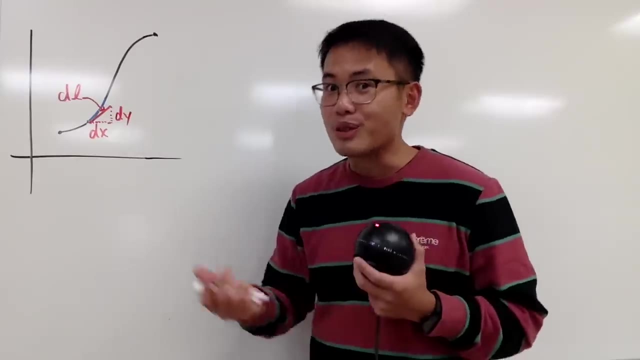 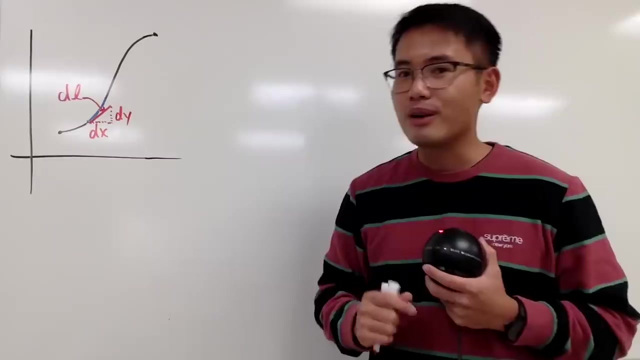 go here and then up, and that will be dy, a small change in the y values. Why do we need dx and dy? Well, because, as you can see, this is where we can do the derivative, And also, by doing that, we come out with a little triangle, little red triangle, so we get to use the 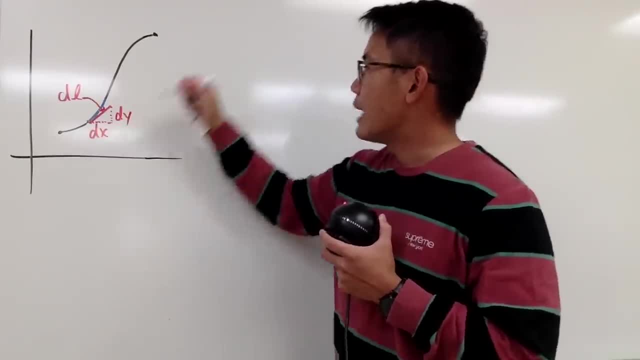 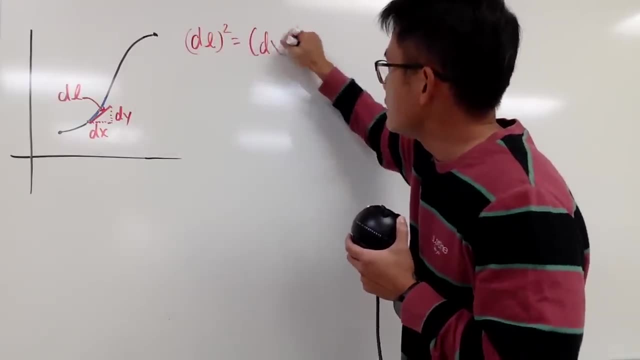 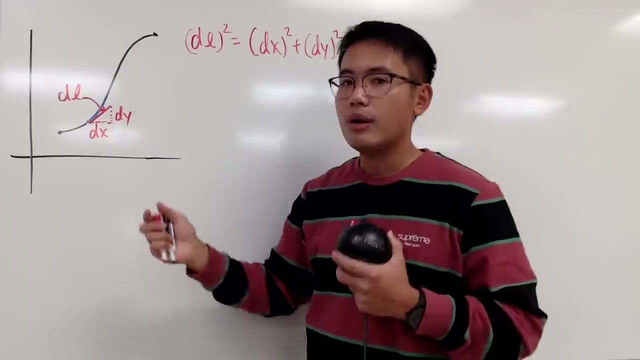 Pythagorean theorem. So, with that being said, we know that by Pythagorean theorem, dl squared is equal to this squared plus dot squared. So let me just write it down as dx squared plus dy squared here, And of course I want to get dl. I can just take the positive square. 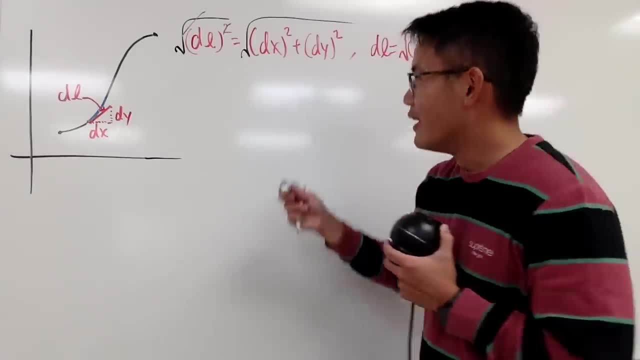 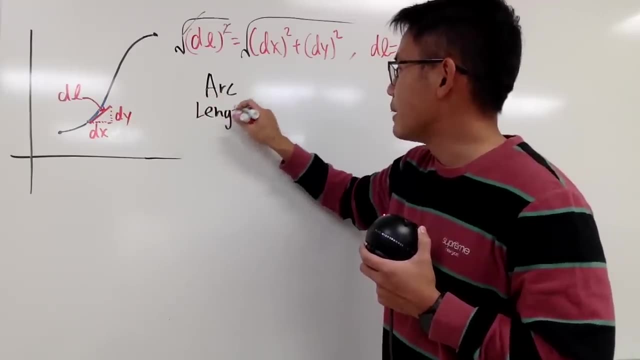 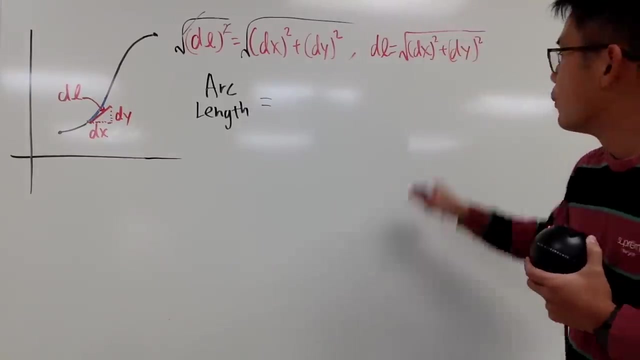 root on both sides. And now here is the deal. For the arc lengths, some books, they put little s for the notations I like to use capital L, but since this is my first video, especially when I'm talking about proof, I would just like to spell everything out. Anyway, here's the deal Once. 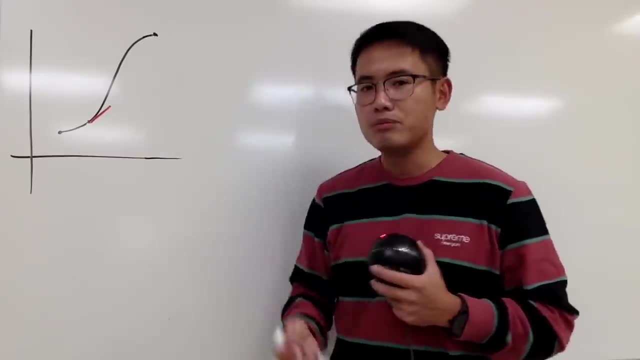 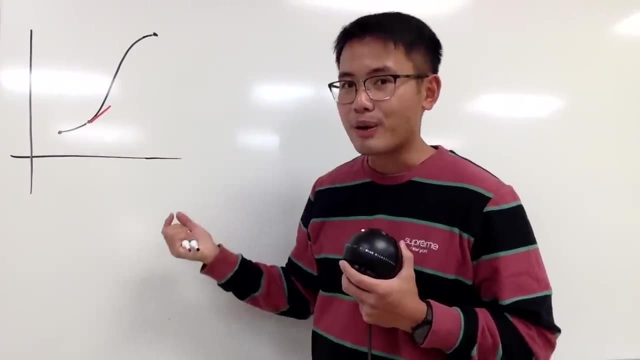 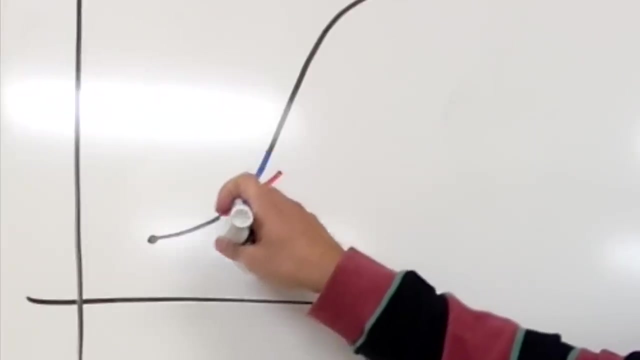 supposed to be really really small, but if I make it so small nobody can see it, so I will just have to make it big. And the idea is that this right here, this length we can calculate it, and this length is going to be really really close to this portion of the arc in blue. 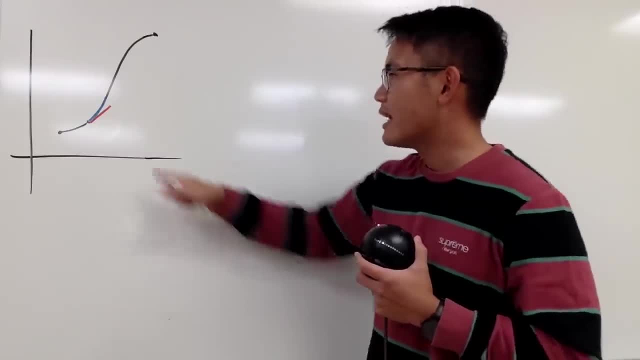 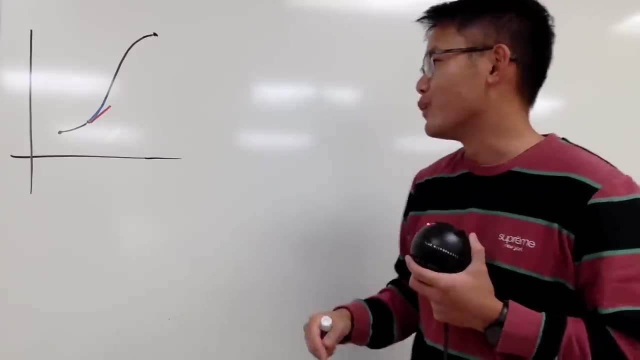 if you make this really really small And the idea is that we'll be using the red part to approximate the blue part and then we'll just add up all the such red part, then we will get the arc length. That's pretty much the idea. 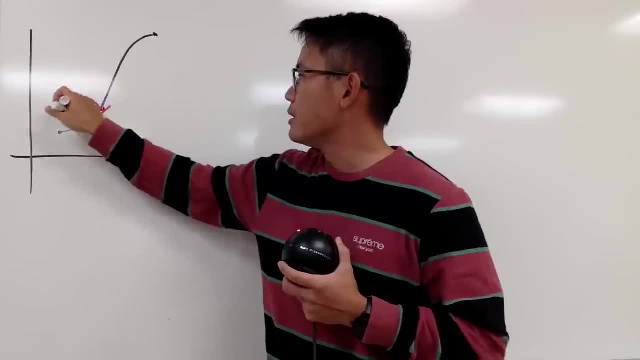 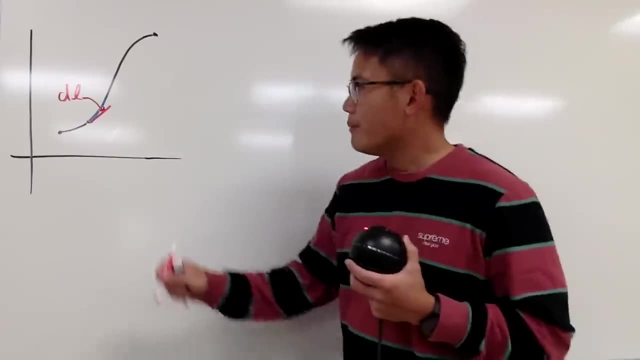 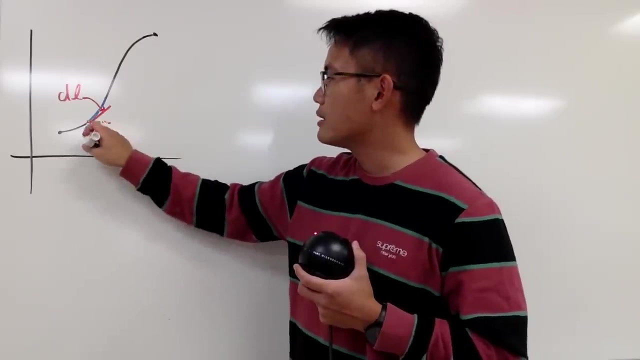 Alright For this. right here I will call it to be dl. Some books call it to be d little s Doesn't really matter. Well, here's the deal. I will actually look at this and I will go horizontally like that, because this right here is the small change in the x values, that is dx. 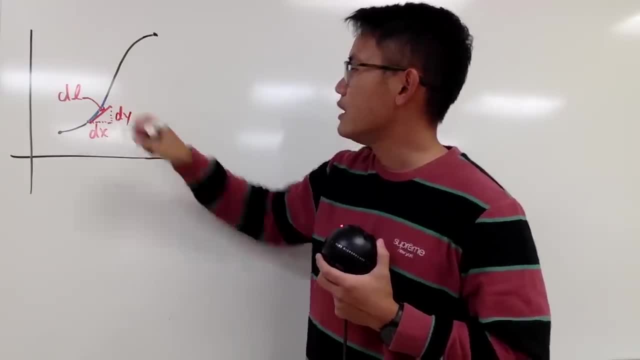 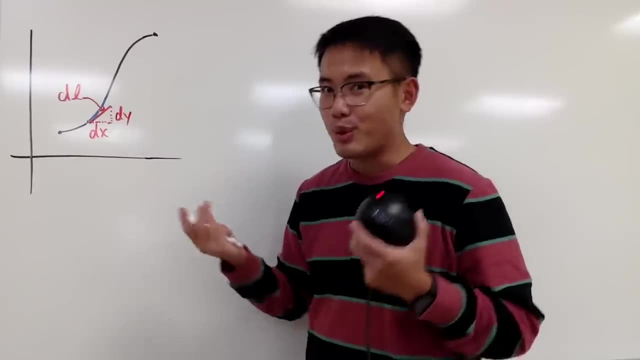 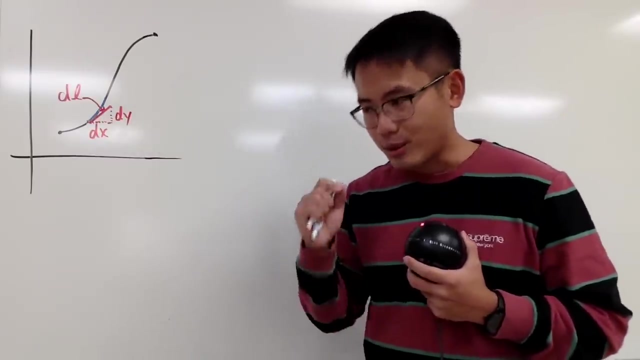 Then I will go here and then up, and that will be dy, a small change in the y values. Why do we need dx and dy? Well, because, as you can see, this is where we can do the derivative, And also, by doing that, we come out with a little triangle, little red triangle. so we get to 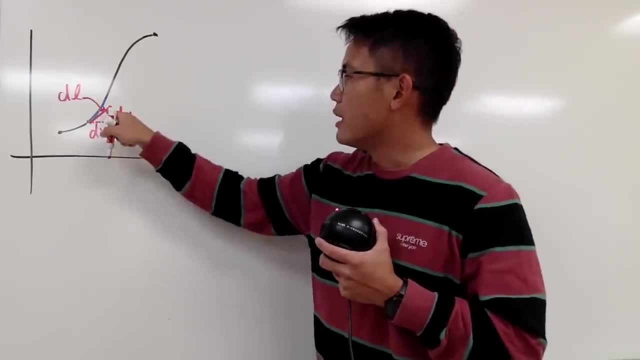 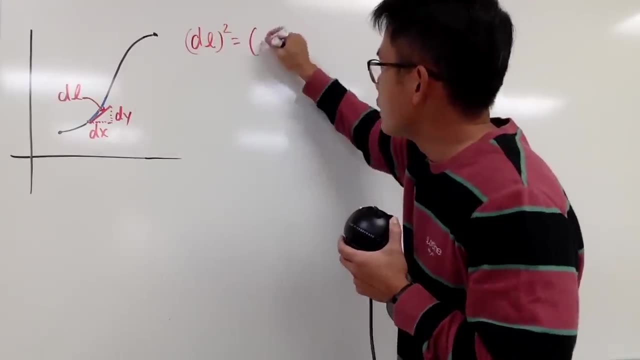 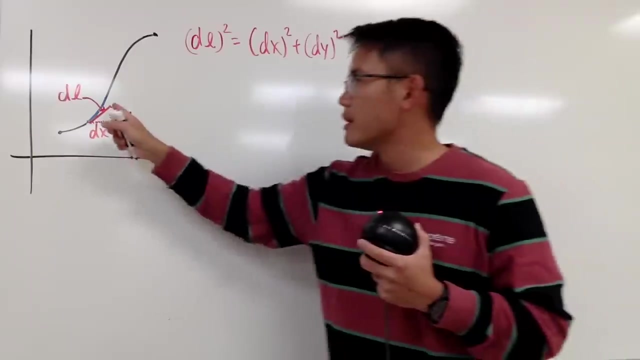 use the Pythagorean theorem. So, with that being said, we know that by Pythagorean theorem, dl squared is equal to this squared plus dot squared. So let me just write it down as dx squared plus dy squared here, And of course I want to get dl. I can just take the positive. 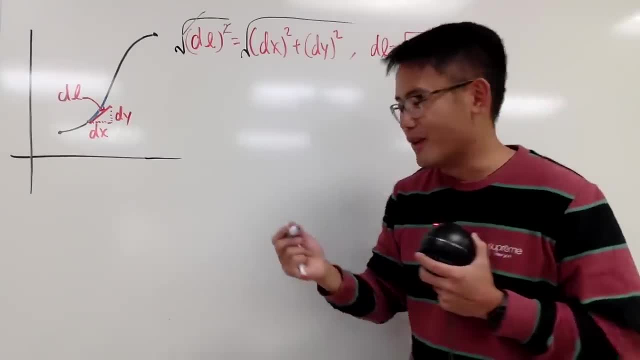 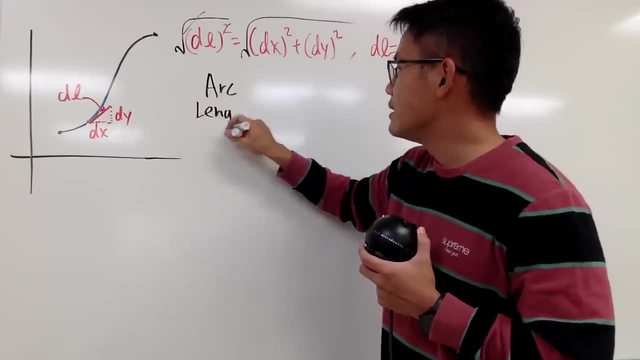 square root on both sides. And now here is the dl For the rth length. some books they put little s for the notations I like to use capital L. but since this is my first video, especially when I'm talking about proof, I would just like to spell everything out. 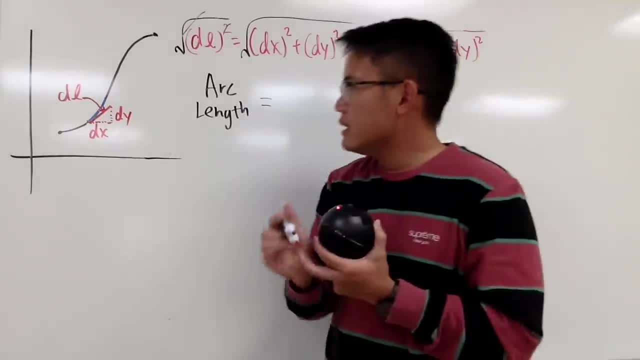 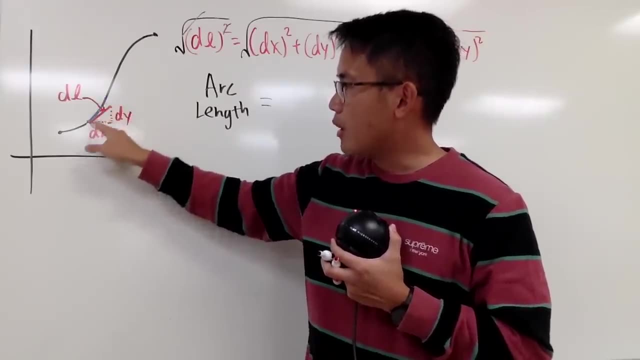 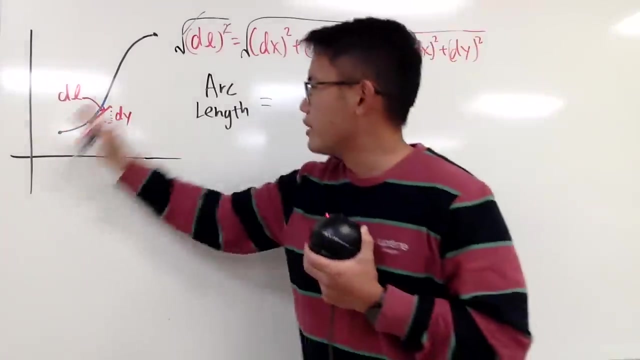 Anyway, here's the dl Once again. this is the dl And this is supposed to be really close to the length of this arc in blue And I just need to add up such little dl. So for the rth length from here to here, it's pretty much that I would. 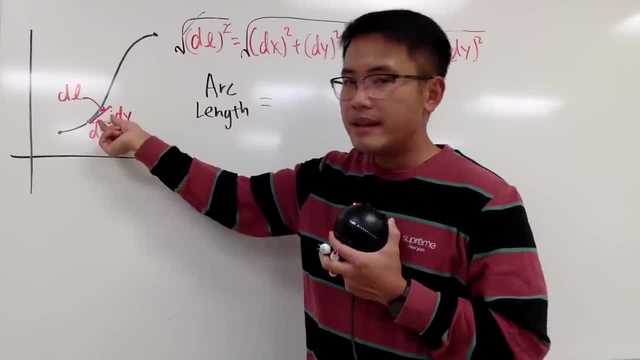 again, this is the dl and this is supposed to be the negative square root of dx. So in the end I will just take the positive square root on both sides and then I will just write it down. So- And this is supposed to be really close to the length of this arc in blue, 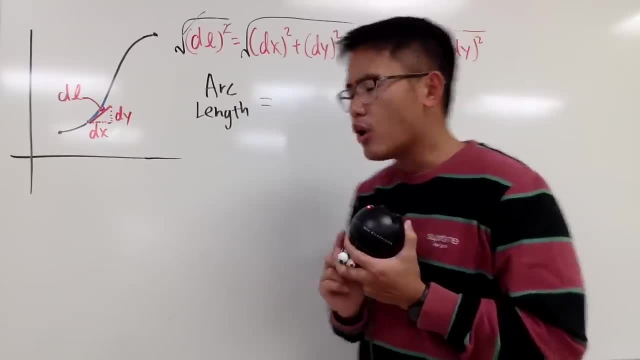 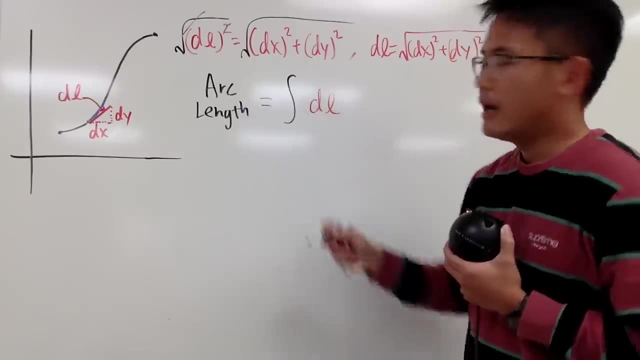 And I just need to add up such little dl. So for the arc length from here to here, it's pretty much that I would just have to do dl and then add them up, and the idea is, of course, use integration. 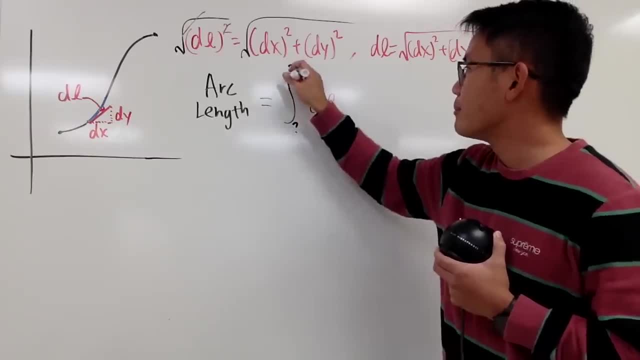 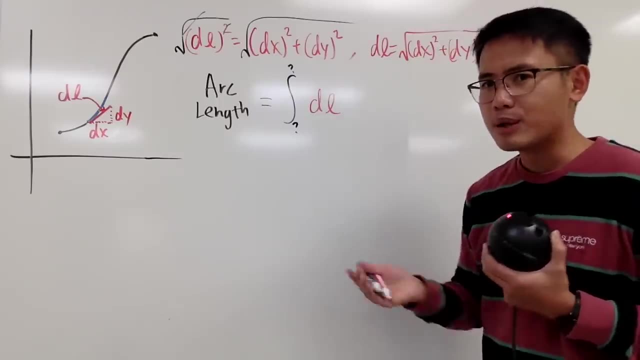 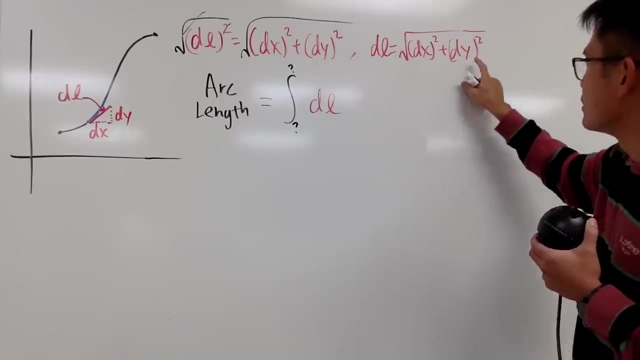 Unfortunately, though, I cannot put down any number here, because I don't know too much about the l world. So we have trouble. and how can we fix that? Of course we have to refer by dl to be this, and you see that we have the dx here and also the dy here. 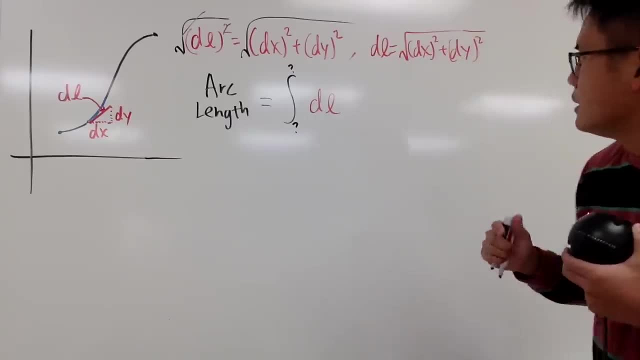 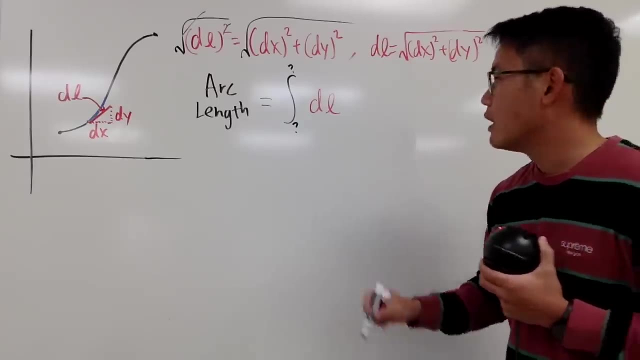 and then, of course, they are being squared instead of the square root. In fact, there are some algebra that we will have to do, and it depends on the situation. Yeah, two situations. The first situation is that maybe this curve right here. 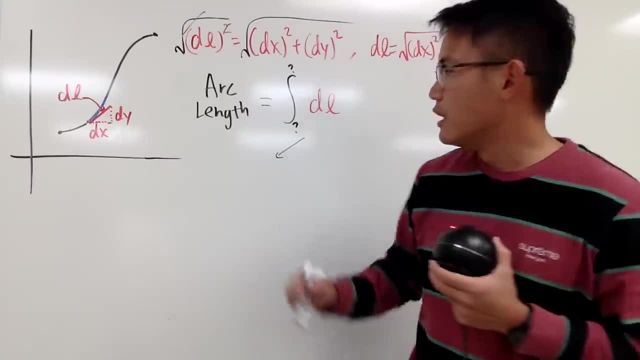 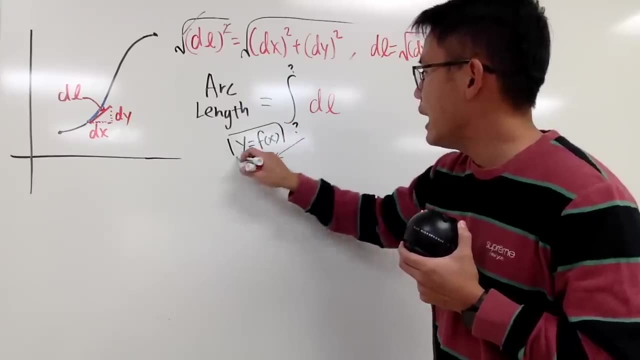 is defined as y to be a function of x, So I will. I will just write down: when we have y to be a function of x, so I'll write it as y equals f of x, Then in that case we do the following: 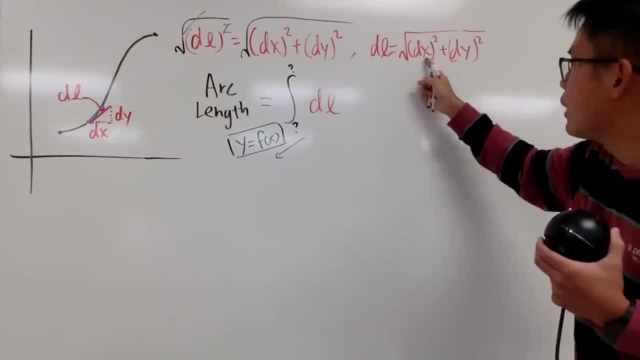 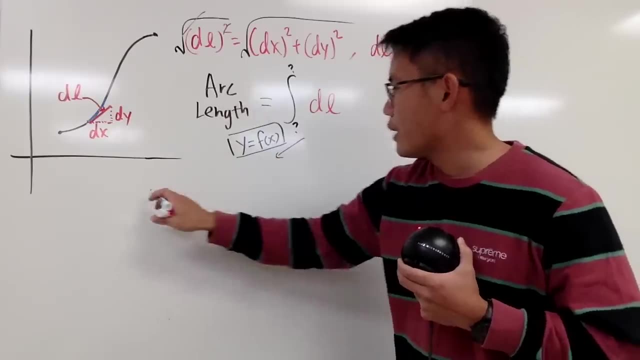 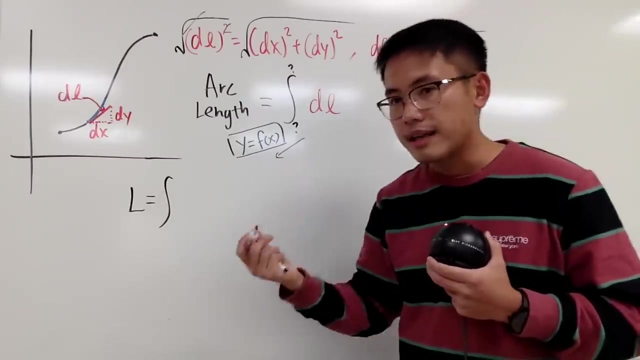 I'm going to look at this expression and I will factor out the dx squared. all right, Let me show you. So this is going to be. I will just put down: l now is the integral, of course, but for the dl, once again, I will factor out the dx squared instead of the square root. 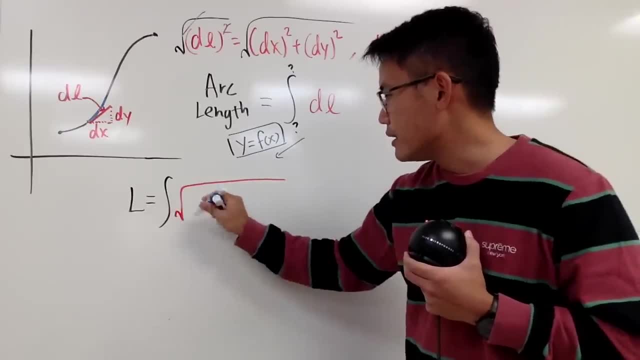 So I will just write down when we have y to be a function of x. So I will just write down when we have y to be a function of x. so let me open the square root first and I will just put down the dx squared first, like that: 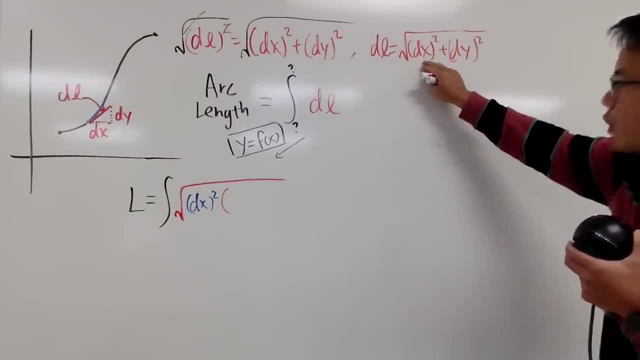 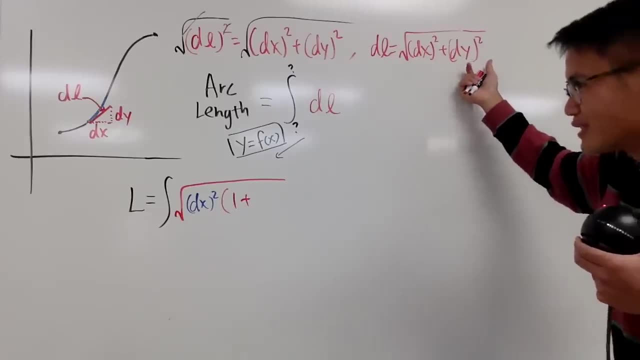 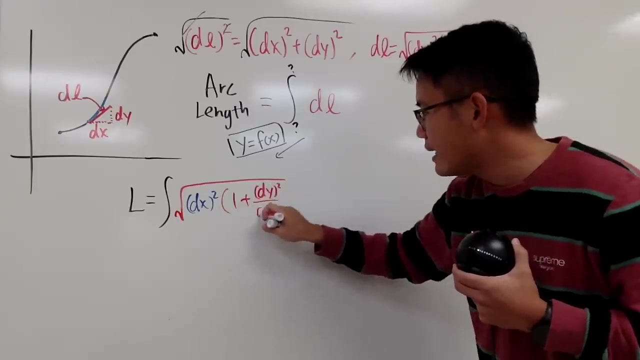 And we will have. Well, originally it was dx squared, but I factored it out already, so that will be 1, and we add it with. This didn't have the dx squared, so I will have to divide. now I will have to put down dy squared and then divide it by the dx squared, like that. 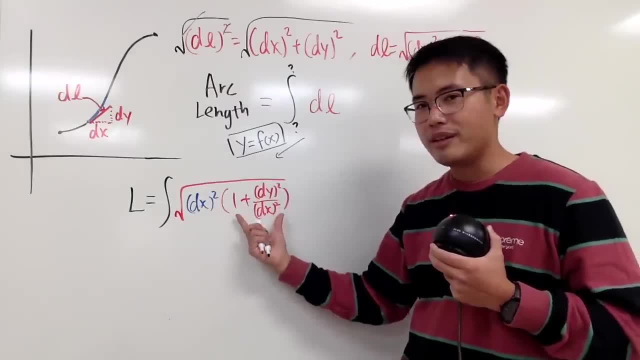 Now you see we have the. Now you see we have the. We have the dx squared times this quantity instead of the square root, so it's pretty much the square root of this times, the square root of that. 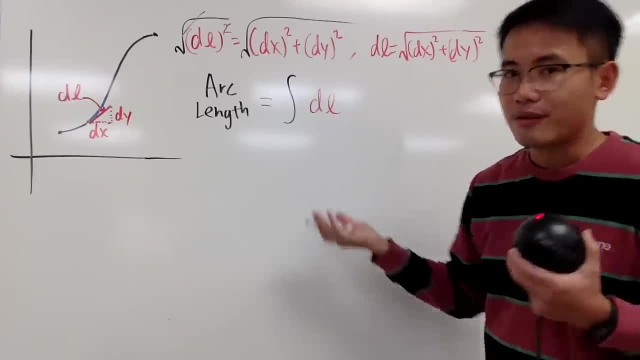 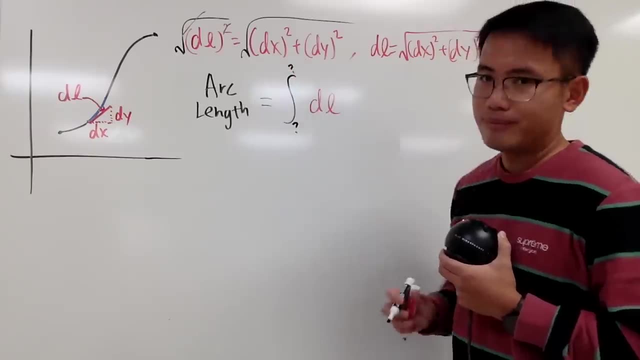 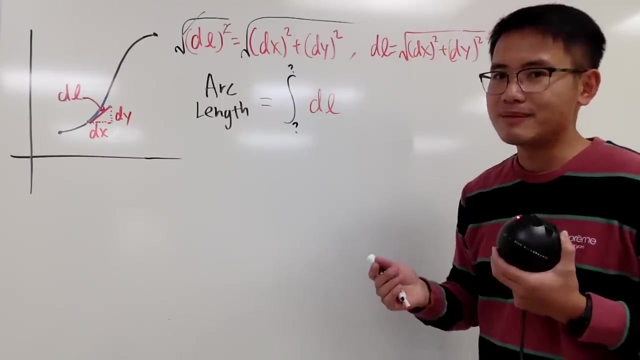 just have to do dl and then add them up, And the idea is, of course, use integration. Unfortunately, though, I cannot put down any number here, because I don't know too much about the L world. So we have trouble. And how can we fix that? Of course we have to refer by dl to be this, And you see that. 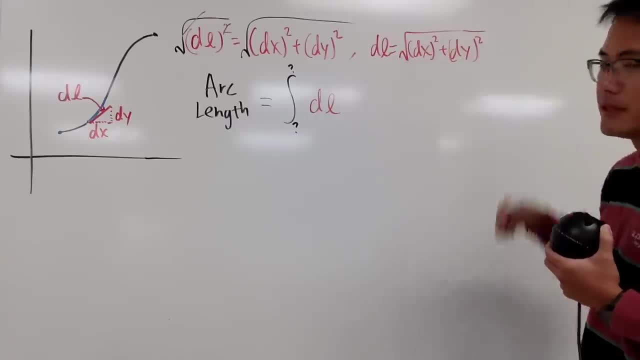 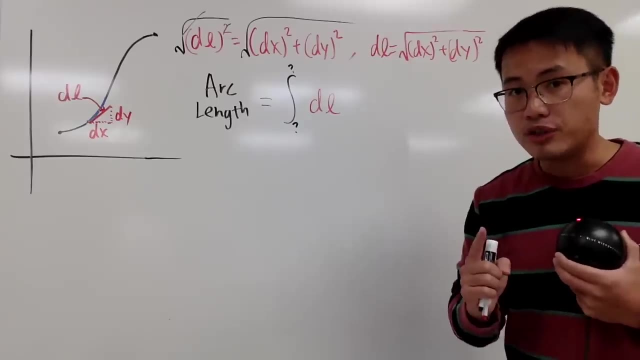 we have the dx here and also the dy here, And then, of course, they are being squared instead of the square root. In fact, there are some algebra that we will have to do, And it depends on the situation. Yeah, two situations. The first situation is that maybe 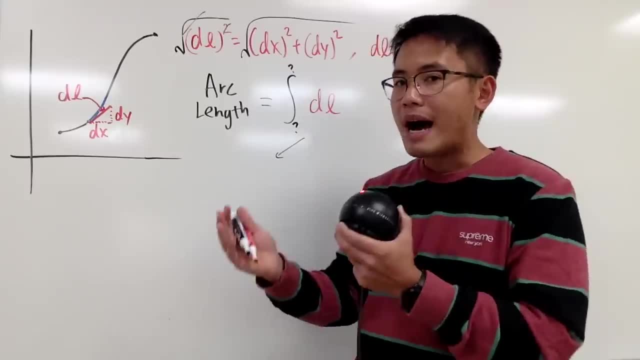 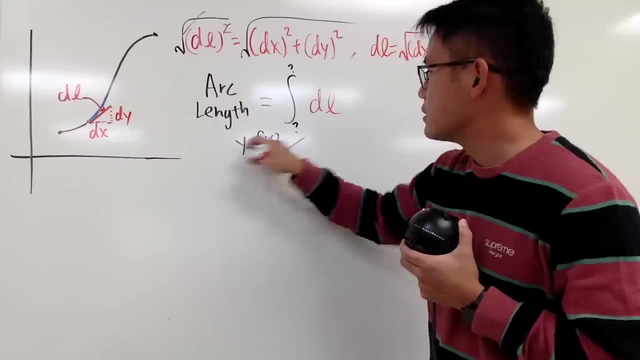 this curve right here is defined as y to be a function of x. So I will just write down when we have y to be a function of x, So I'll write it as y equals f of x, Then in that case we: 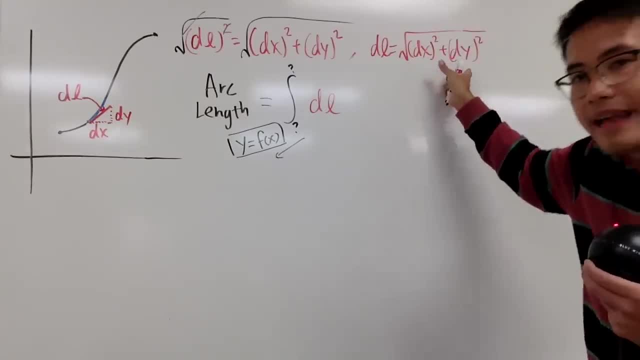 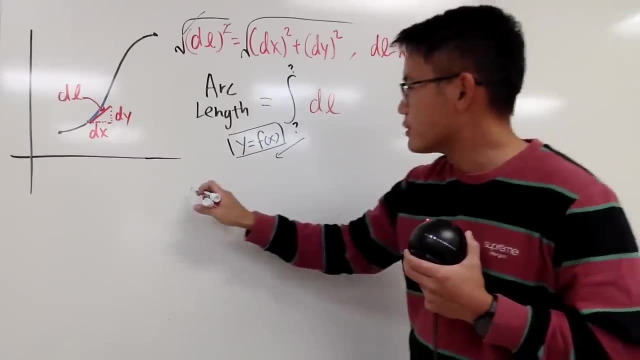 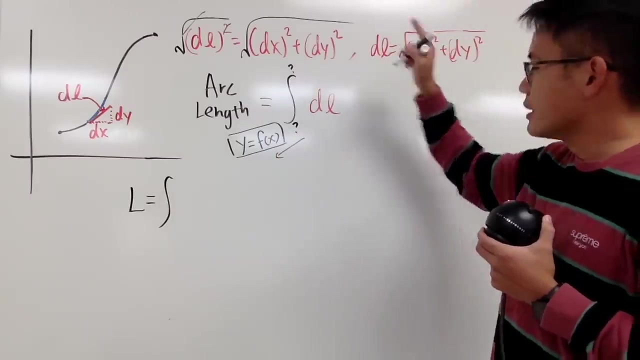 do the following: I'm going to look at this expression and I will factor out the dx squared. Let me show you So this is going to be. I will just put down: L now is the integral, of course, But for the dl, once again I will factor out the dx squared instead of the square. 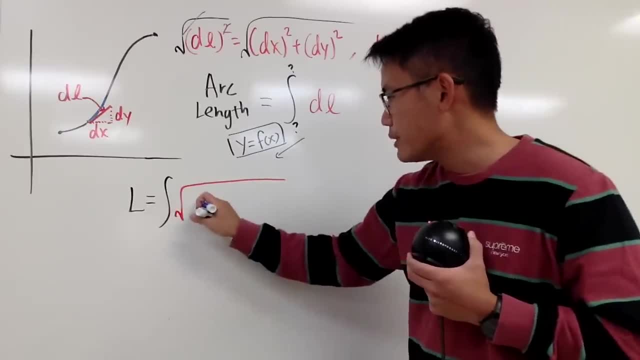 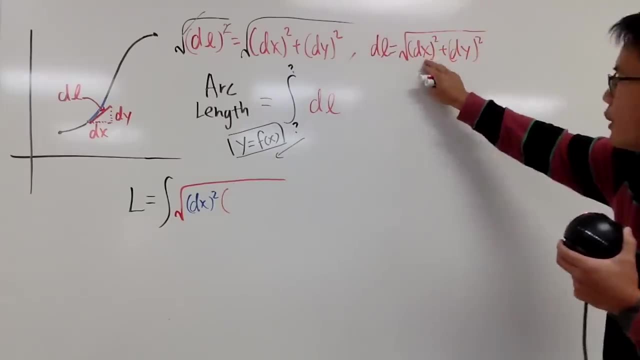 root. So let me open the square root first And I will just put down the dx squared first, like that, And we will have. well, originally it was dx squared, but I factored it out already, so that will be 1. And we add it with this: 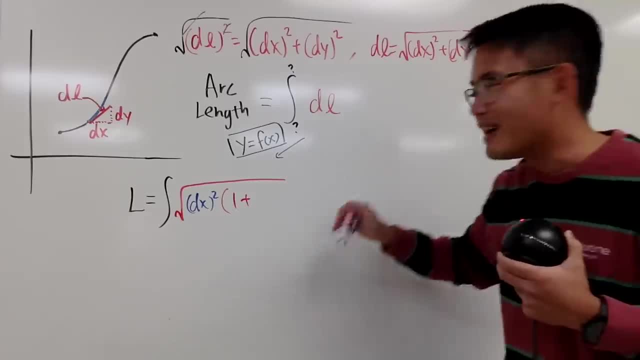 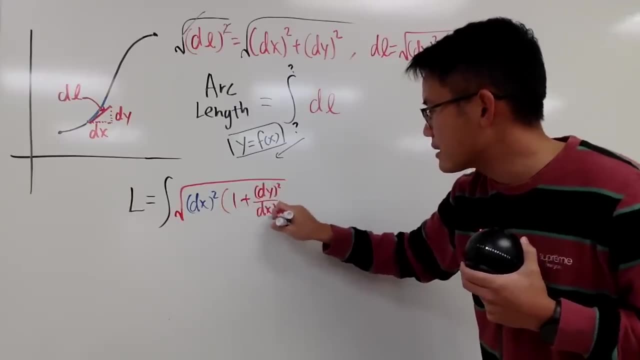 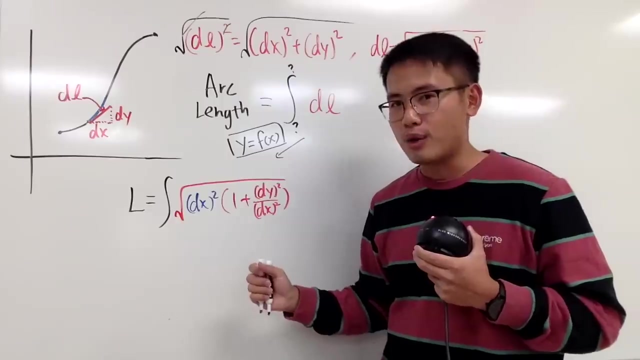 didn't have the dx squared So I will have to divide. now I will have to put down dy squared and then divide it by the dx squared, like that. Now you see, we have the dx squared times this quantity Right. So, as you can see, we have a constant right And the took forward from the circle. 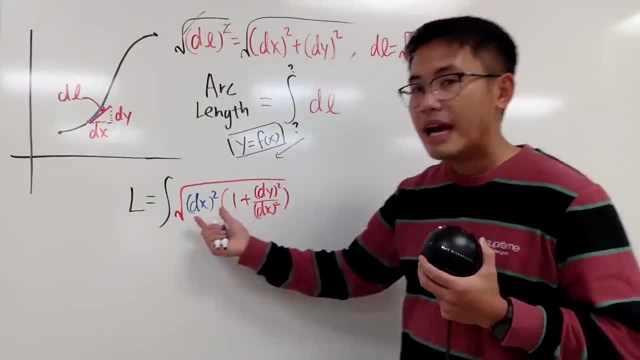 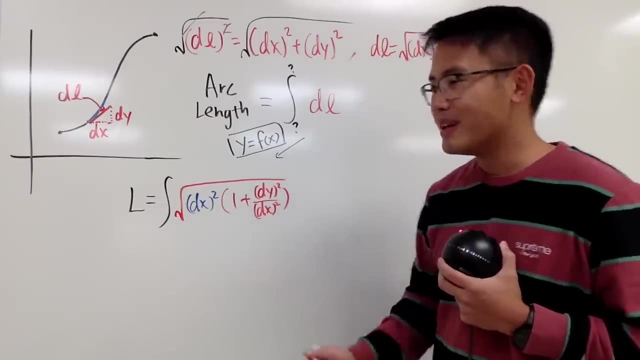 is the integral. So 1 and 1, this is the integral. So the integral is going to be the integral of the integral of the integral, and that's going to give us, for our whole equation, the integral at the end of the integral. And from here you see the square and the square. 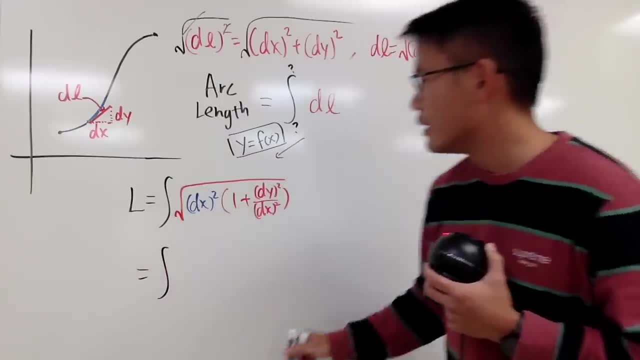 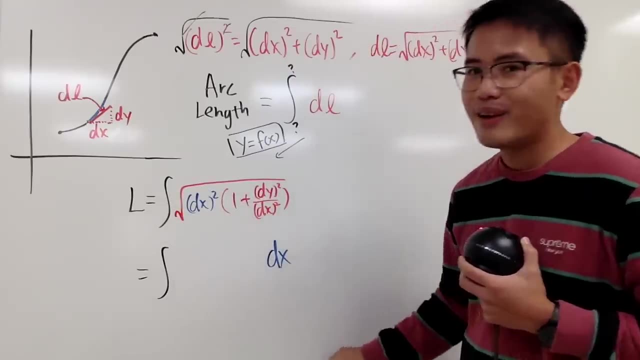 will cancel and we just get the dx And we can put that at the end of the integral And I'll write it down for you guys. This is the integral And this is going to give me just the regular dx. I will put that at the end, right here. And for the integral. 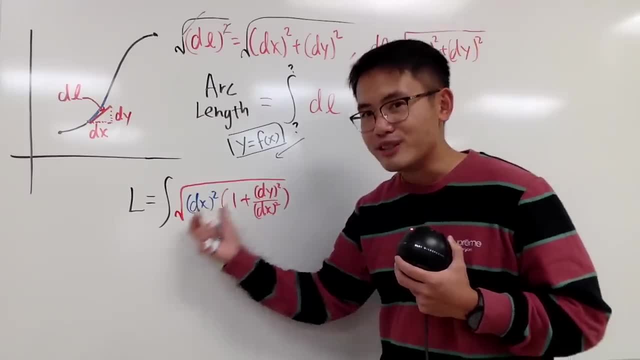 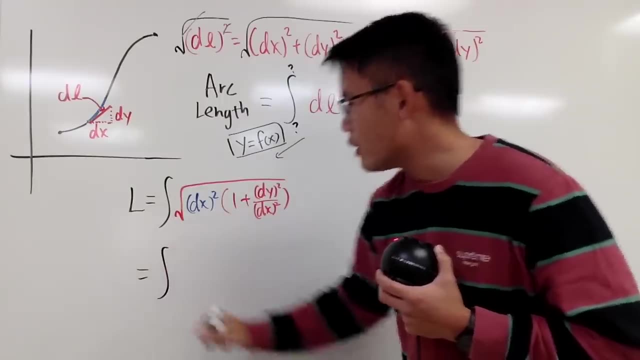 And from here you see the square and the square root cancel and we just get the dx and we can put that at the end of the integral And I will write it down for you guys. This is the integral and this is going to give me just the regular dx. 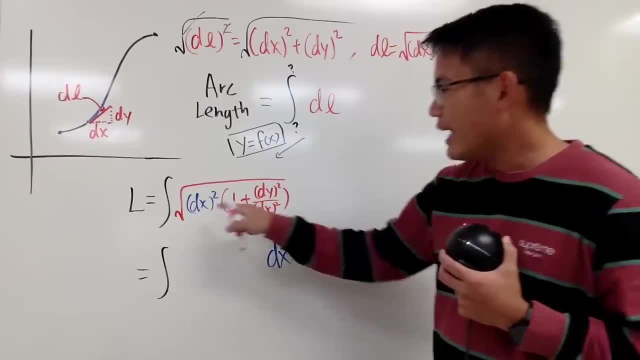 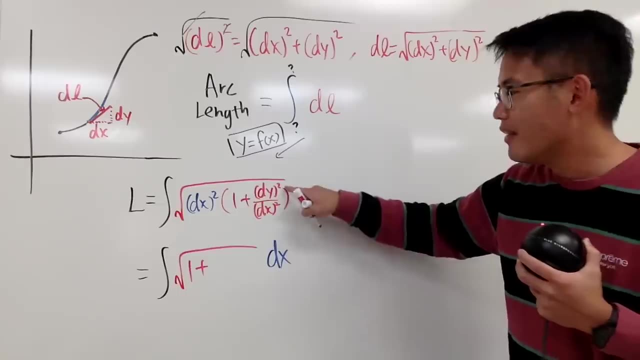 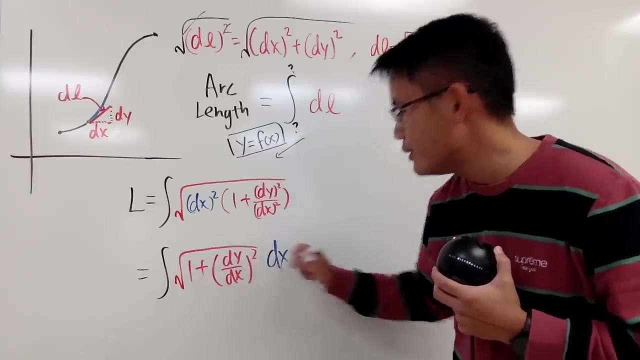 I will put that at the end, right here, And for the integral it's just the square root of 1 plus, and notice that they are both to the second power, so of course we can write it as dy, dx and then you square. 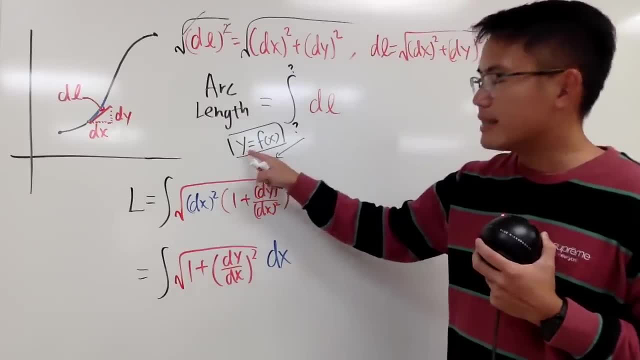 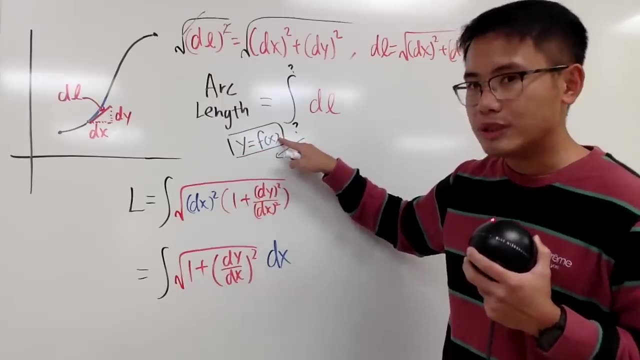 And here's the deal For the dy dx. you are going to look at this equation: differentiate y with respect to x, Namely you do the derivative right here with respect to x, Get the derivative, put it here square, that add a 1,. 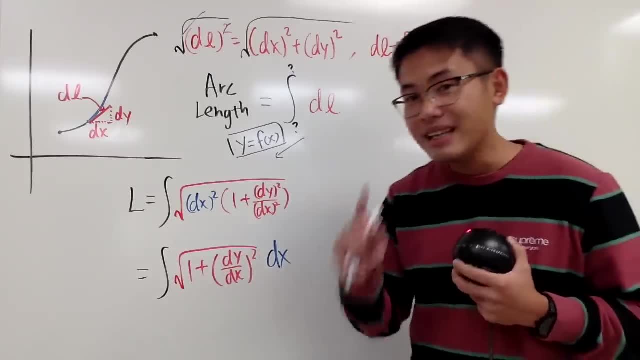 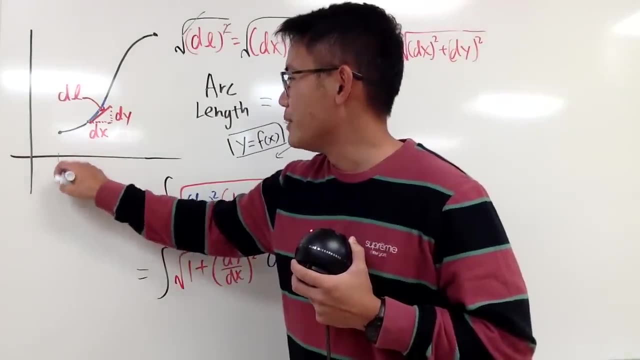 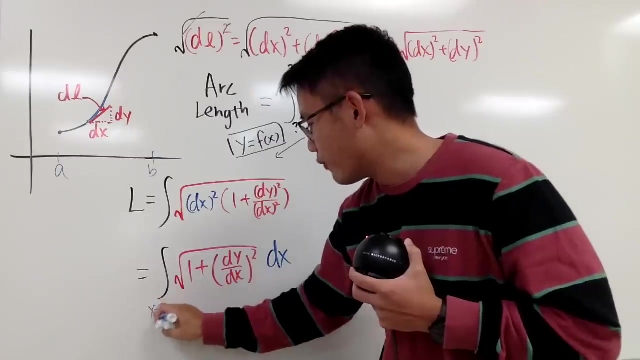 put it in the square root, dx. and because you're in the x-world, go back to the picture, look for the x-value and I'll just call the x-value to be a to b, like that. So, with that said right here, you know you will have to go for a to b. 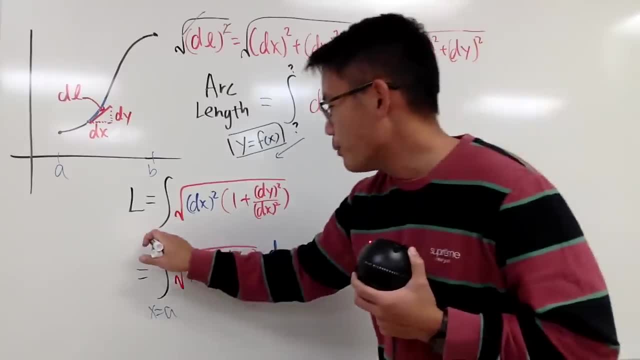 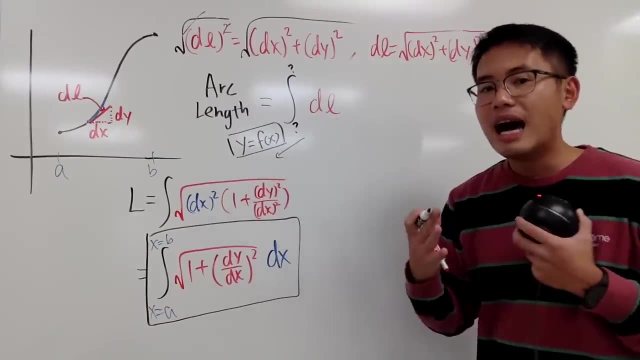 and that's the x-values. So this is the Ard-Lang's formula, the first version, and you use this when you have y as the function of x. On the other hand, if you were given x as the function of y, 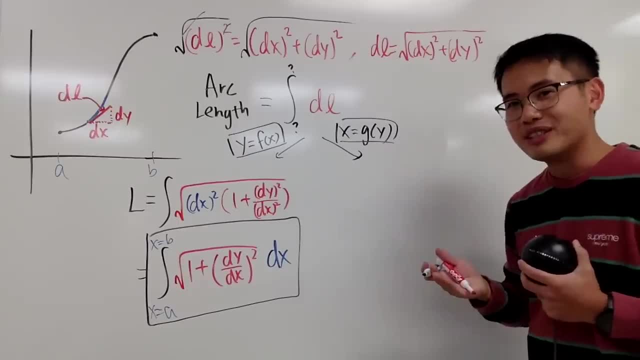 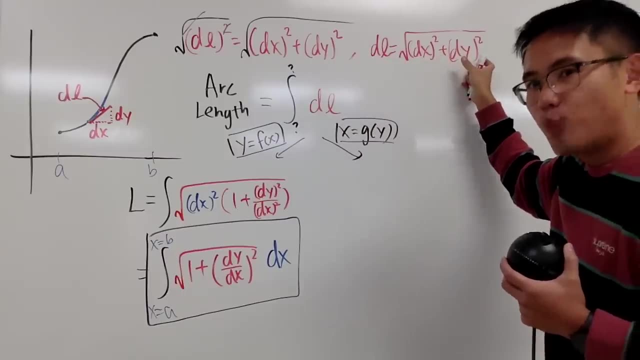 really similar to the previous video. we may have this situation as well, and in this case for the dl part. I'll be looking at this and then factoring out the dy squared instead of the dx squared, So it's pretty much like the opposite of that. 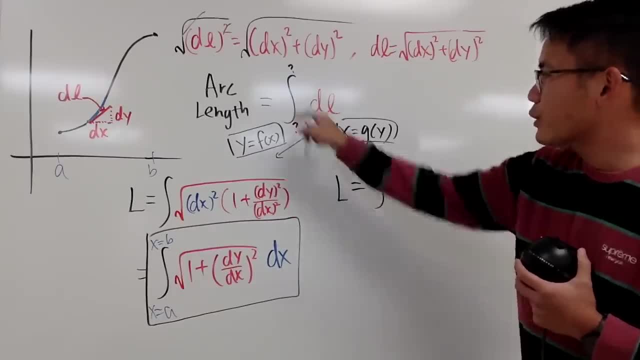 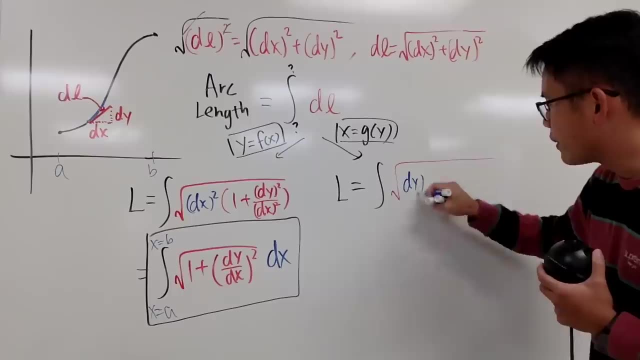 And now let's get to work. We'll write down: l is equal to integral and for the dl, you open the square root first and then we'll factor out the dy squared. put it here first and then from here we get this term. 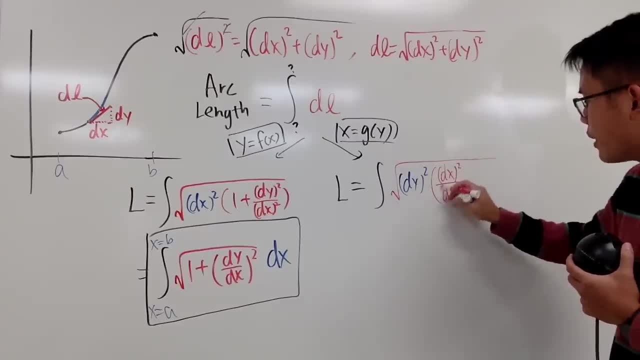 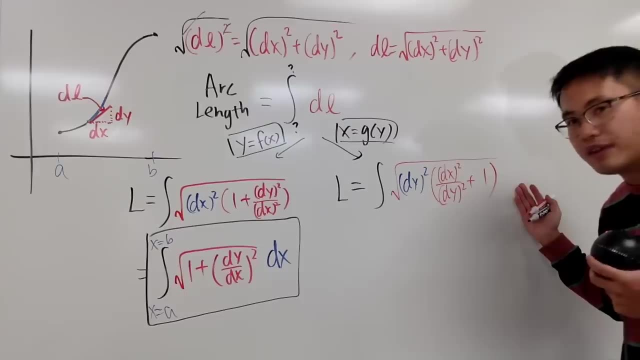 it's going to be dx squared over dy squared, and then we add it with: this is going to be just a 1. And do not put down dy right here, because we don't have any Like this. we didn't have any. 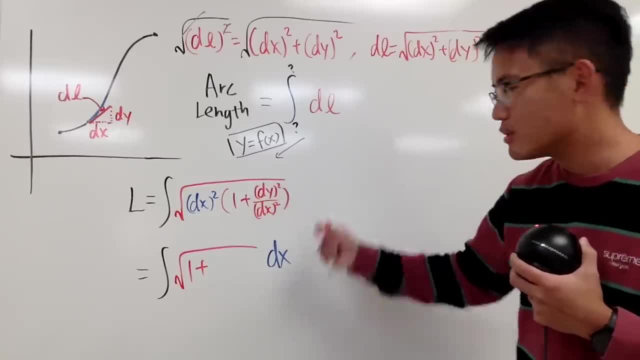 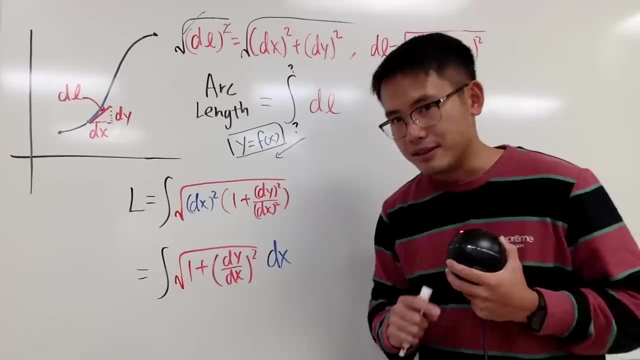 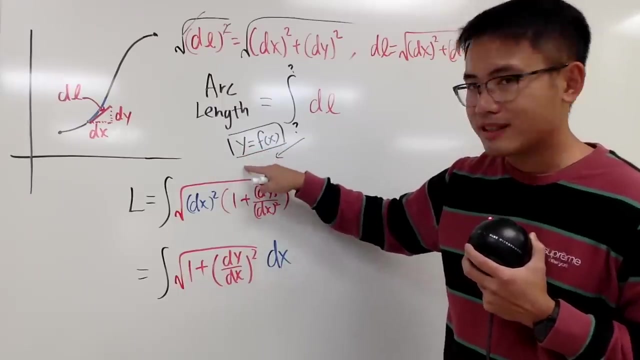 And notice that they are both to the second power. so of course we can write it as dy dx. and then you square, And here's the deal For the dy dx. you are going to look at this equation: differentiate y with respect to x. 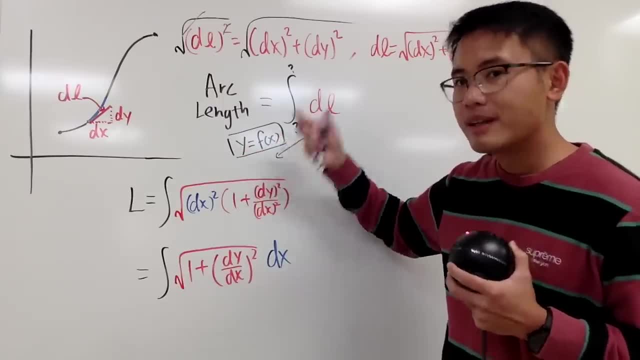 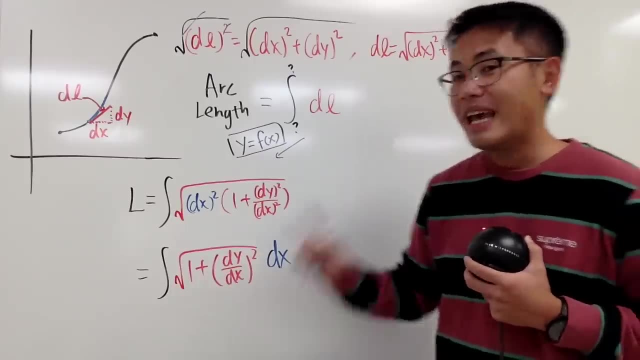 Namely, you do the derivative right here with respect to x. Get the derivative, put it here, square that. add a 1, put it in the square root dx. and because you're in the x world, go back to the picture. look for the x value. 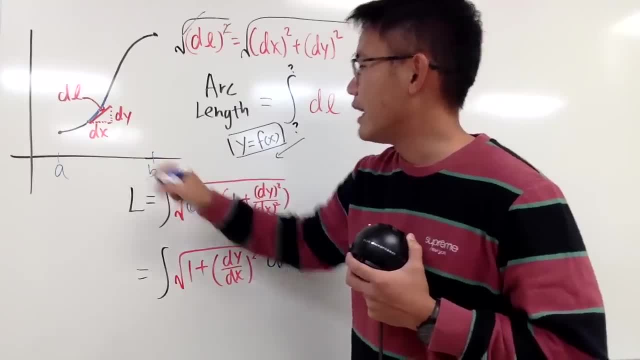 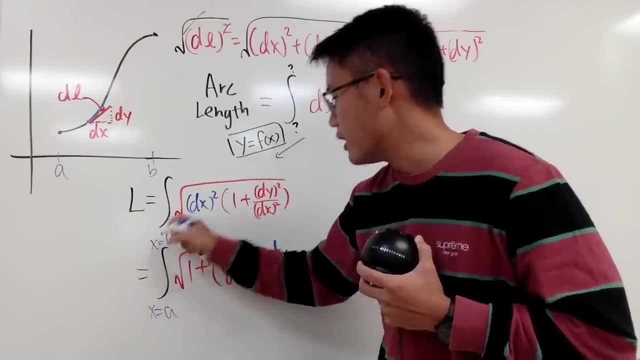 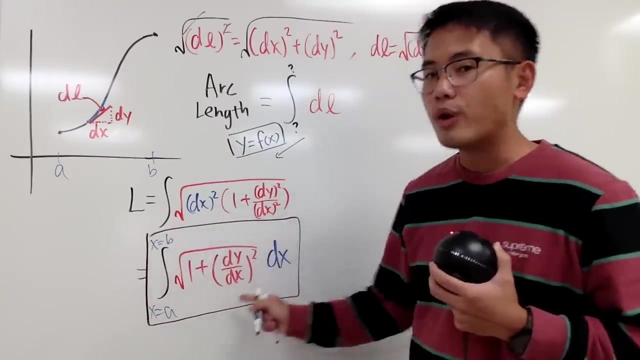 and I'll just call the x value to be a to b, like that. So, with that said, right here, you know you will have to go for a to b and that's the x values. So this is the Archling's formula, the first version, and you use this when you have y as the function of x. 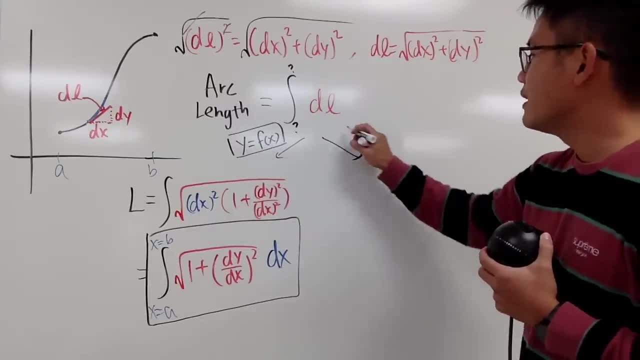 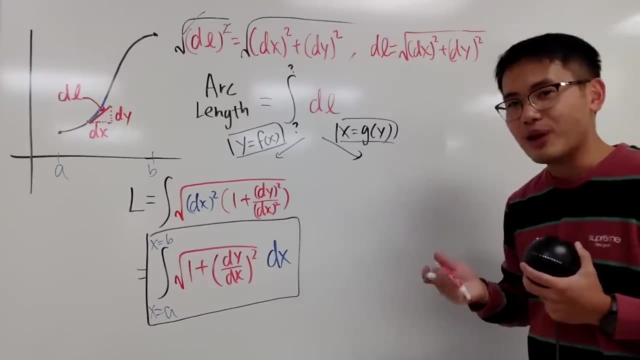 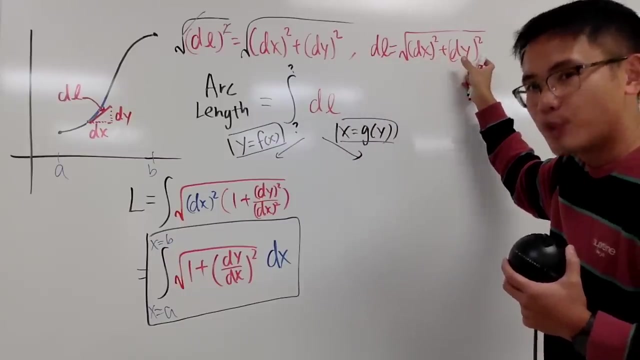 On the other hand, if you agree, So this is given x as the function of y. Really similar to the previous video. we may have this situation as well, And in this case, for the dl part, I'll be looking at this and then factoring out the dy squared instead of the dx squared. 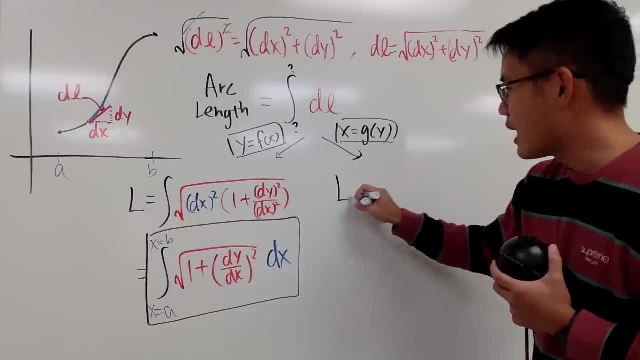 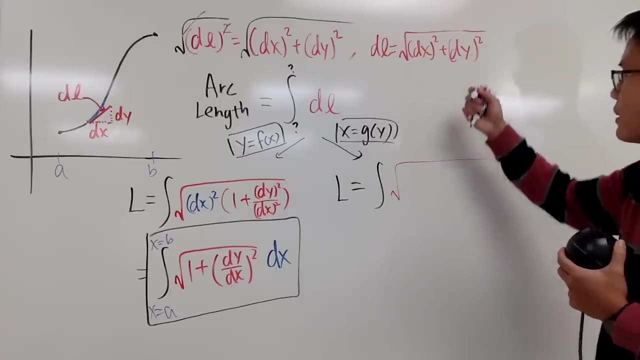 So it's pretty much like the opposite of that. And now let's get to work. We'll write down: l is equal to integral and for the dl you open the square root first and then we'll factor out the dy squared. put it here first. 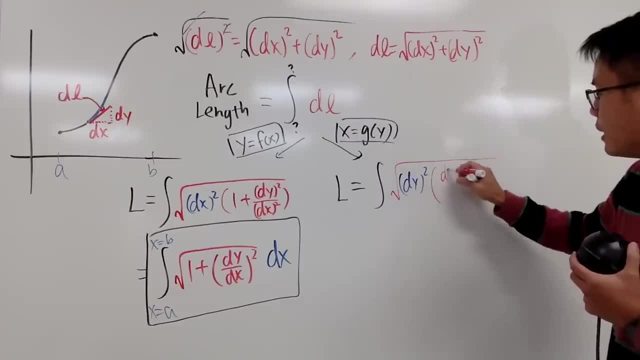 And then from here we get this term. it's going to be dx squared over dy squared, and then we add it with: this is going to be just a 1.. And do not put down dy right here, because we don't have any. 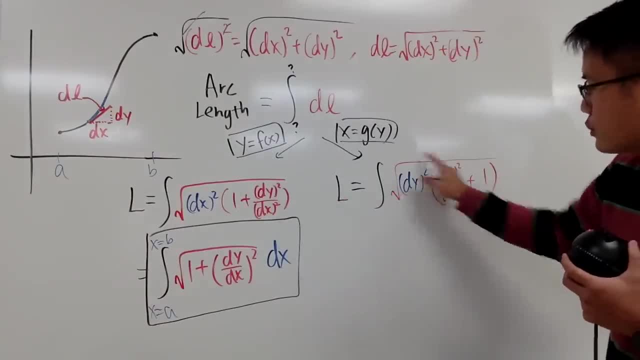 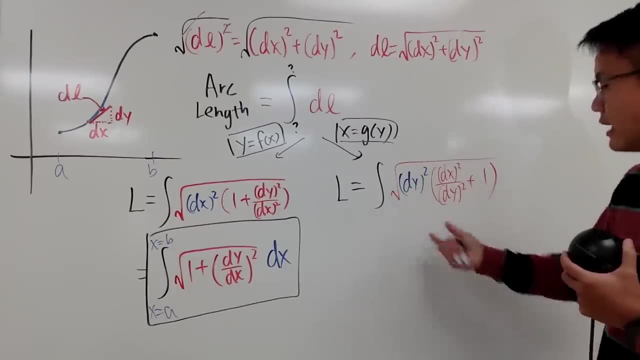 Like this. we didn't have any Look at. this is square root of dy, squared, squared and square root cancel. so this becomes the dy at the end and then we have the square root of this as the integral. So in the end you see that l is equal to the integral. 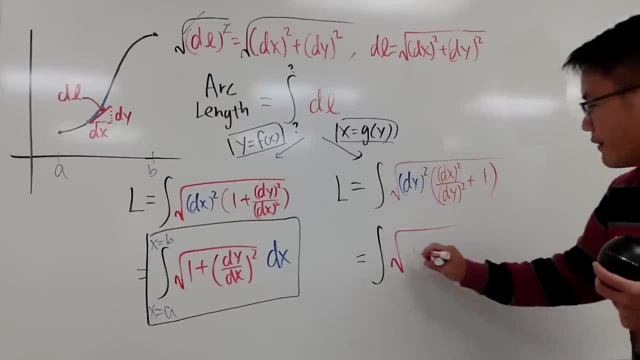 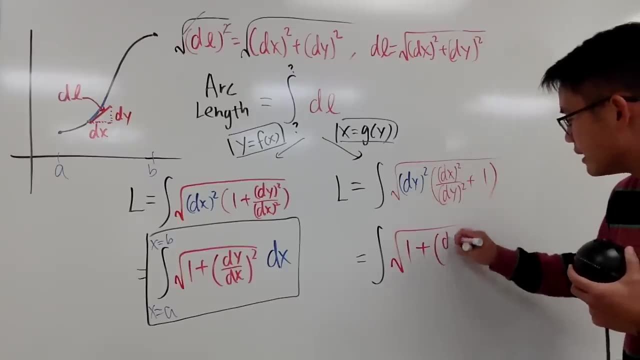 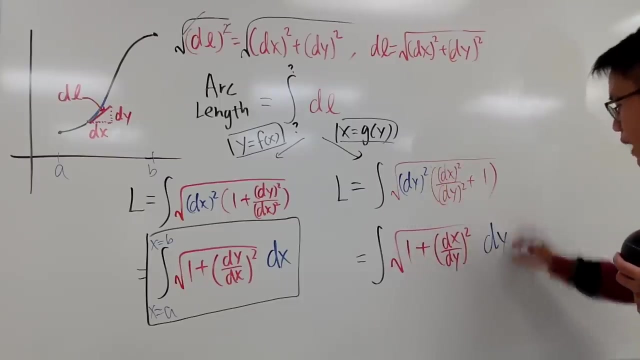 the integral in the square root. and let me put down the 1 first. And we will be adding with this: dx squared over dy squared, we can write it as dx, dy and then you square that and this right. here is the dy at the end.